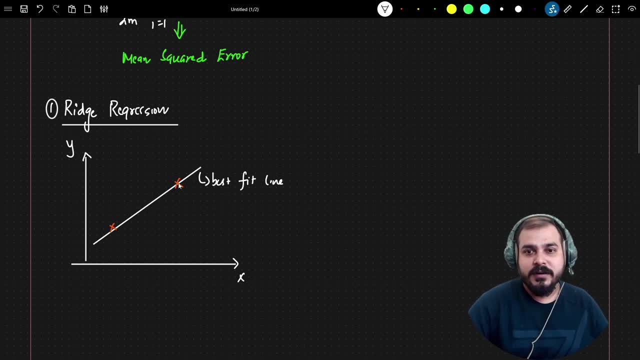 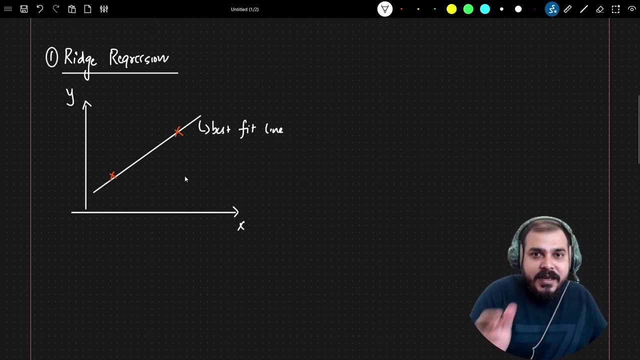 error is zero right, Because there is no such difference right Between the predicted and the real point. So in this particular scenario, I can definitely say this model is overfitting. Now, what does model overfit basically mean? Okay, now with respect to this training data. 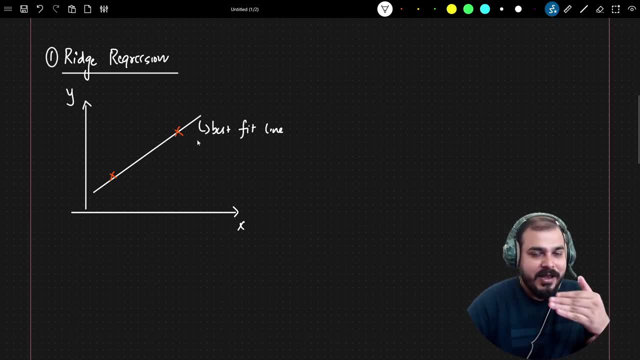 you can see that the accuracy is very high. The error is very, very less right. Error is almost zero right. But if I try to add some more new test data, let's say these are my new test data to add over here Now, when this new test data is basically getting added, you can see that now the 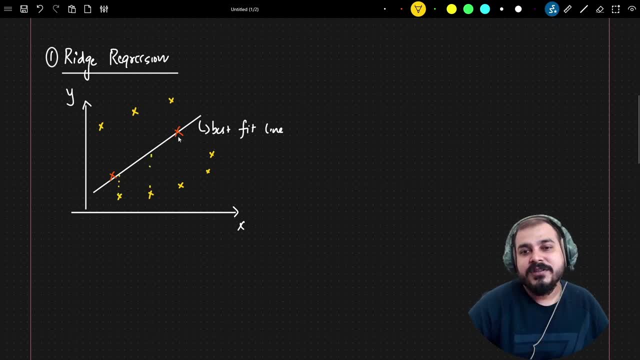 error basically increases. right, The error with respect to this new test data is basically increasing. So this is basically a problem of overfitting. So here, what is actually happening? Here overfitting is actually happening. Now, what does overfitting basically mean? 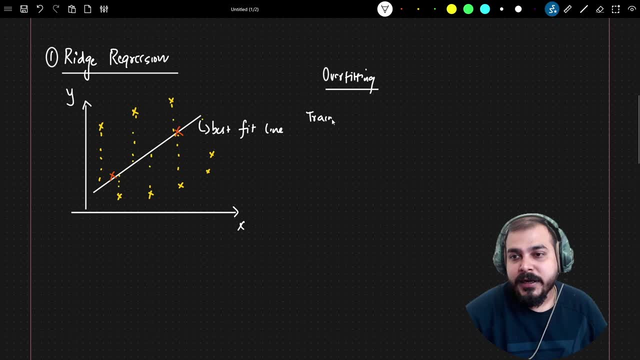 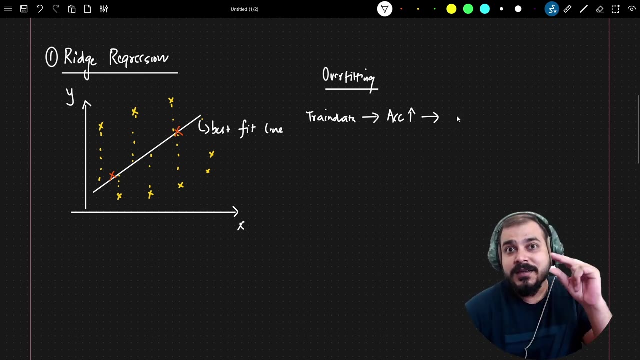 Because I have already covered this. Let's say, with respect to our train data, my accuracy is very, very high. Let's say, my accuracy is 99 percent or 100 percent. okay, And whenever I talk about train data, at that point of time we use something called as bias. 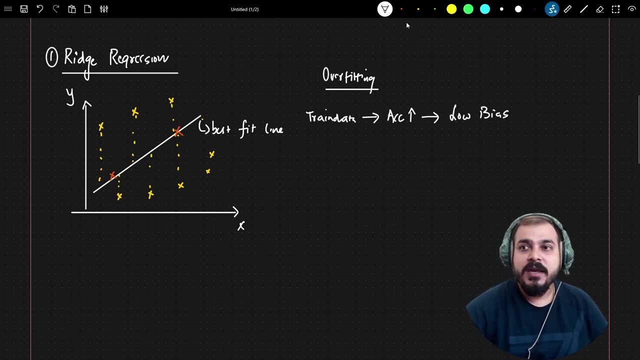 In this scenario I will be saying low bias, okay. Similarly, with respect to the test data, when my accuracy is actually low: see for the train data, the accuracy is high, but for the test data over here the accuracy is low. And in this, 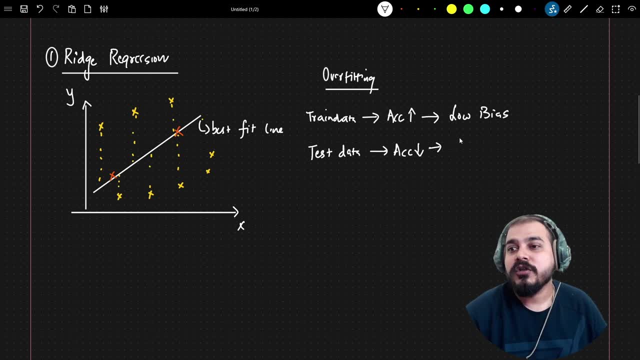 scenario: whenever we use test data. here I'm actually going to use something called as variance, And in this scenario it will be high variance, okay, So this is the problem. that is basically happening, right? It is overfitting in this scenario, right? 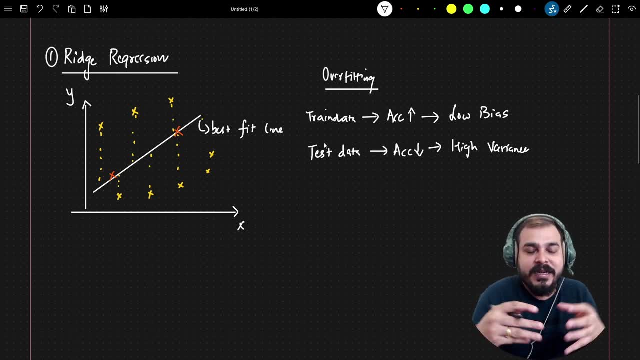 Now, how do I reduce this overfitting? I should definitely find out a way to reduce this overfitting and for that specific scenario we use called as ridge regression, Because in this scenario I know my best fit line is passing through both the points. 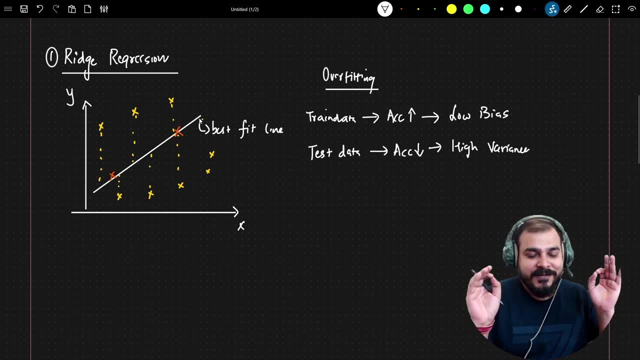 points. okay, and always remember, guys, if you get an accuracy of 100 percent right, definitely consider it that the model is overfitting. you should never get the training accuracy as 100 percent. let's imagine this. that basically means the model has been trained very well on the 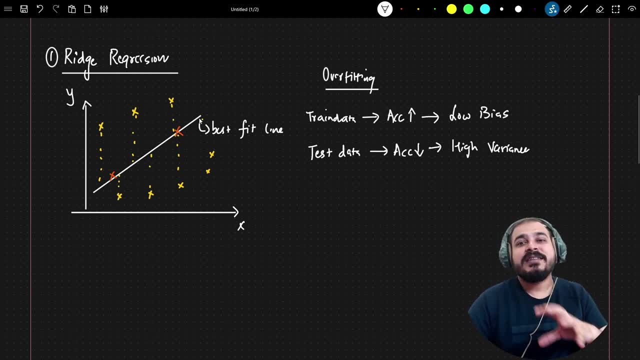 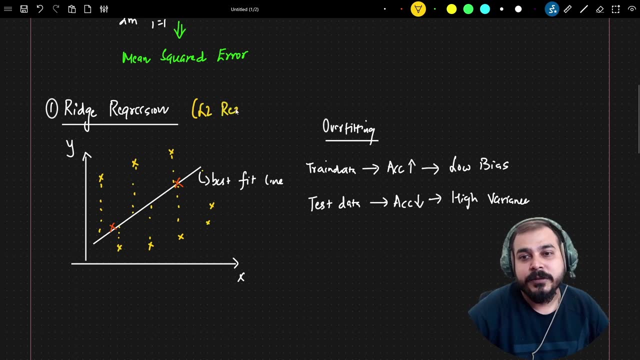 training data. right now, let's understand what exactly ridge regression is all about. okay, ridge regression is also called as something called as l2 regularization- l2 regularization- and this is used to reduce overfitting. suppose my linear regression creates some overfitting, then in order to reduce that overfitting in the linear regression, 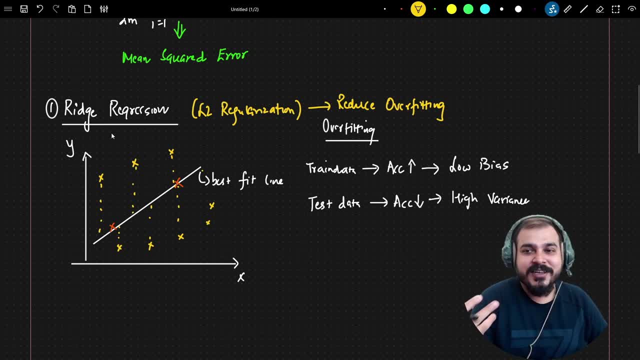 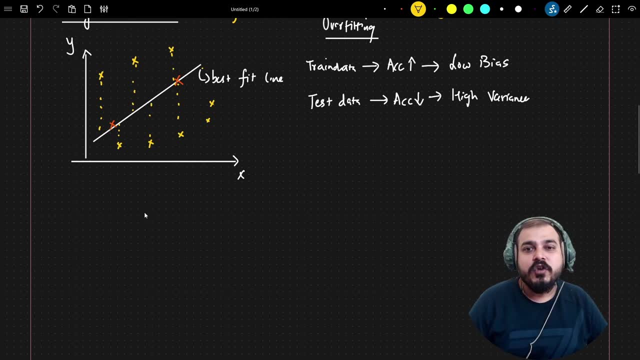 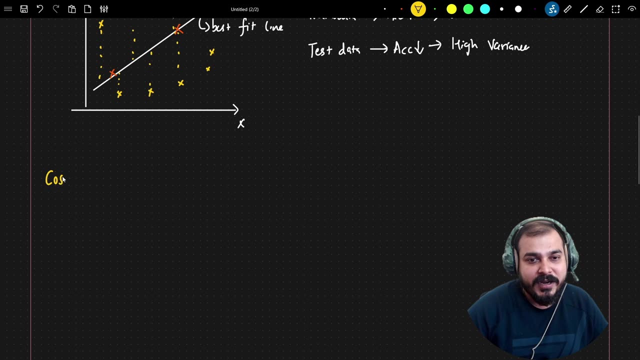 we use ridge regression. okay, so we can just consider ridge regression as a new algorithm which will actually help us to hyper parameter tune the linear regression, okay, okay, now let's go ahead and let's understand. how does the cost function with respect to ridge regression look like? so here i'm just going to write down the cost function. initially, if i 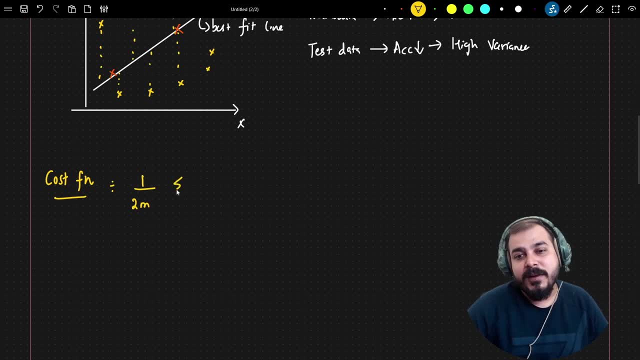 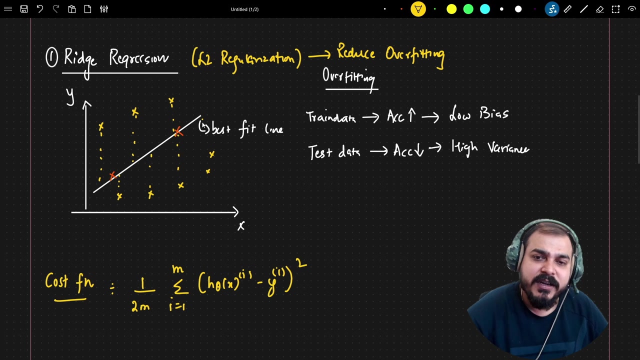 consider the cost function of linear regression. i hope everybody knows 1 by 2m summation of i is equal to 1 to m, h theta of x of i minus y of i, whole square right. so this is the cost function of the linear regression. now, in this particular case, see when i create this best fit line: it. 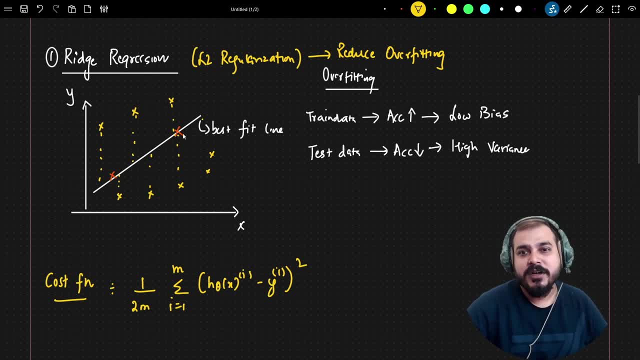 automatically, you know, passes through both the points, both the points in my training data. now, when this is the scenario, obviously my entire cost function. this will become zero. right now, when it is becoming zero, that basically means my model is overfitted because it is passing through all the points. 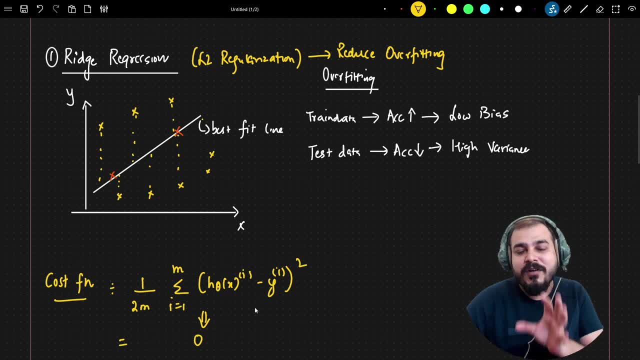 perfectly. now, in order to you know, remove or add some parameters, that we have to make sure that this never becomes zero. so what we do is that in ridge regression, we add two parameters: one is lambda and the other one is lambda and the other one is lambda and the other one is lambda and the. 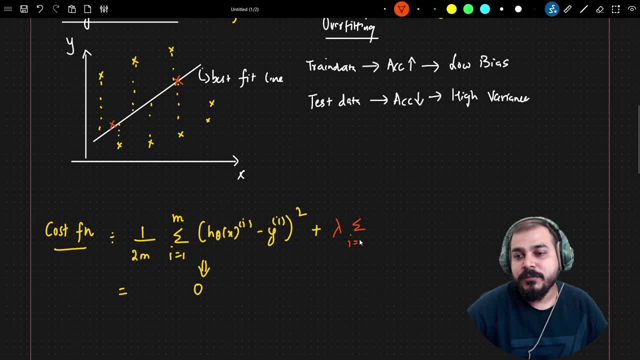 second one that we try to add is: summation of i is equal to 1 to m slope square. okay, so this lambda that you see is a kind of hyper parameter. okay, and i'll try to show you the relationship between lambda and slope and how this is basically reducing the overfitting. that also will try to. 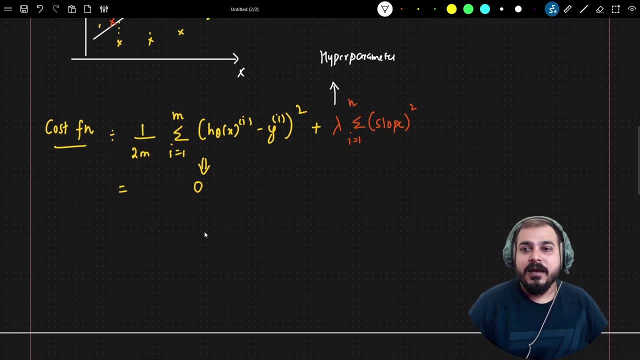 understand. okay, now see over here if i am trying to add lambda and slope square. let's say lambda value is one. okay, now when this value becomes zero, i have to make sure that this never becomes zero, because if this becomes zero, that basically means this best fit line perfectly passes through all. 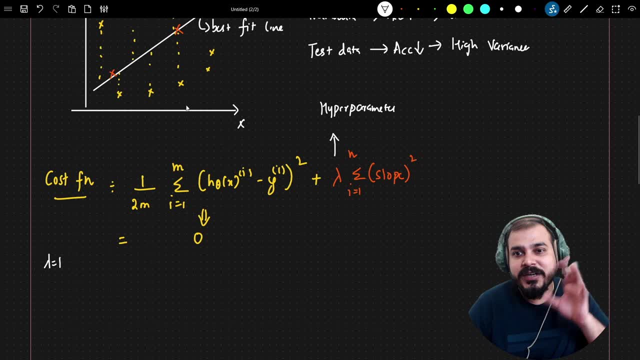 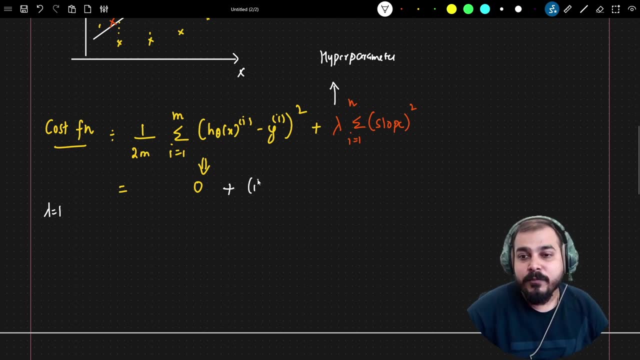 the points, and this should not happen. so my cost function should definitely know that this is not zero at this point of time. so what we do, we do we penalize this value by multiplying one lambda value. lambda value, i've just initialized as one, okay, and then i'll try to show you the relationship. 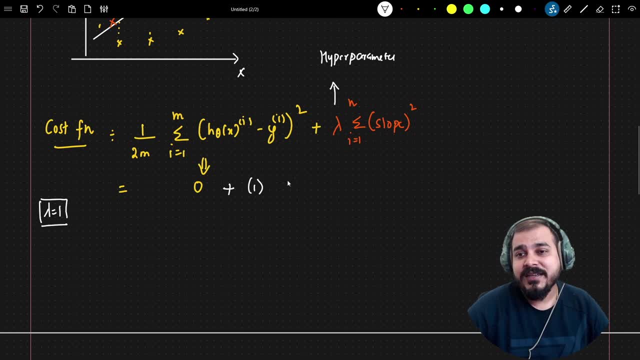 between lambda and slope. so after this one, let's say my slope, my, in this particular case my h theta of x is nothing but theta 0 plus theta 1 x 1. okay, let's say i just have one input features. so summation of i is equal to 1 to m, basically means how many. 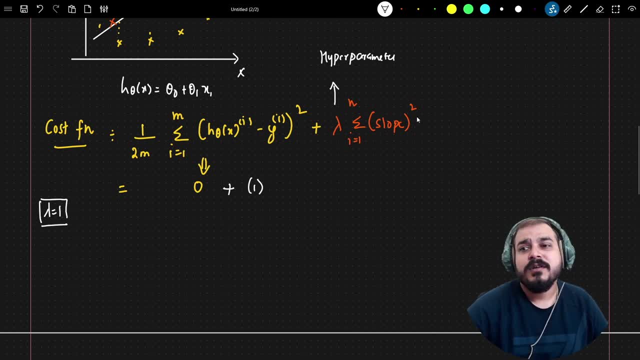 number of coefficients or slopes are there. we are just going to do the summation of whole square, like that. so here i'm just going to do theta 1, whole square. now let's consider theta 1- any positive or negative value, okay, so that basically means we are never going to get zero. we will be. 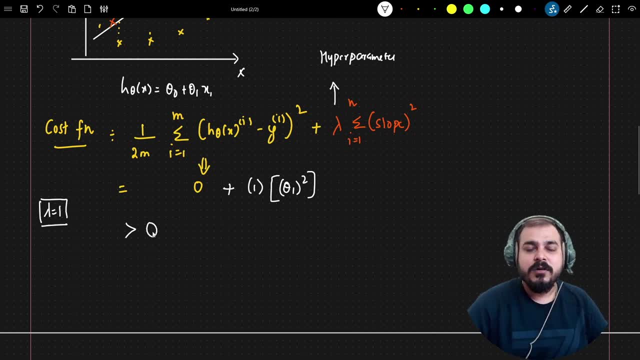 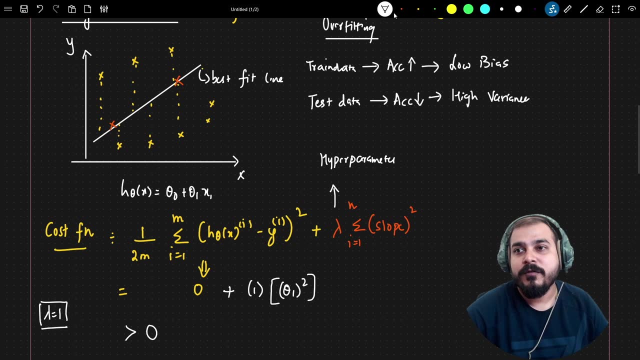 getting greater than zero right in this particular scenario, what will happen is that my model training the best fit line will just not get stopping, not just stop over here. then it will try to find out another best fit line like this, or it will try to find out another best fit line like this, such that my cost function is 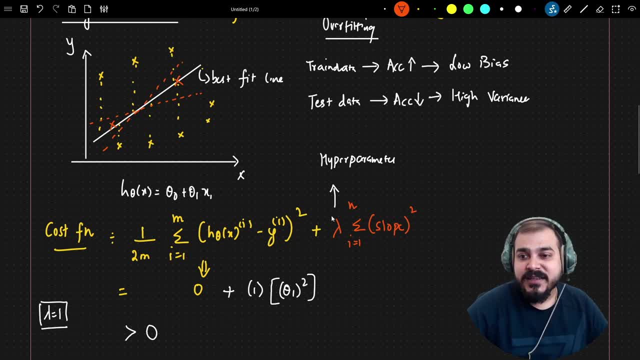 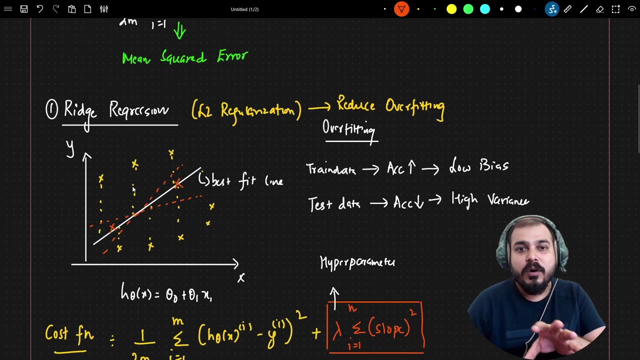 minimal. okay, so in this specific way, when i am specifically adding these two parameters, that is, lambda and slope square, the situation is going to be in such a way that we are never going to get a best fit line that passes exactly through all the training data points. okay, so this is how ridge regression. 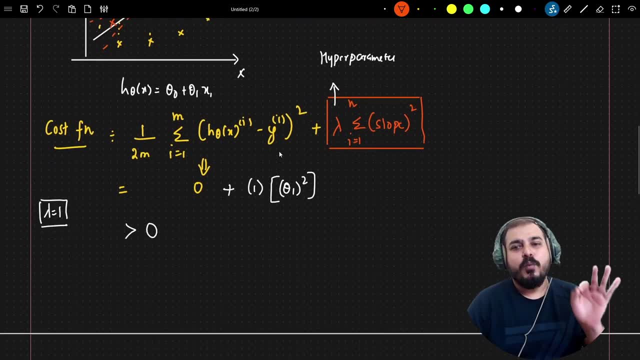 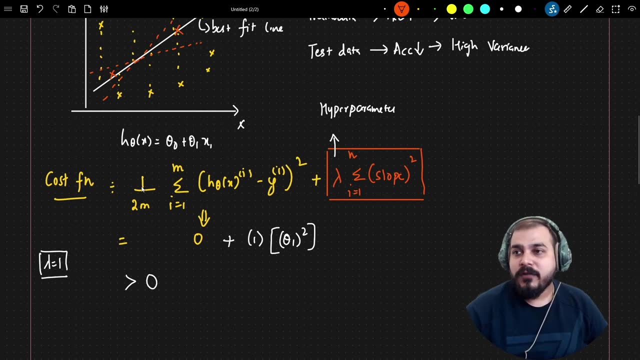 is making sure that the overfitting will not happen. but one very important interview question that may come: what is the relationship between lambda and slope square? okay, and for this let's draw that same curve that we discussed, you know, with respect to the simple linear regression. 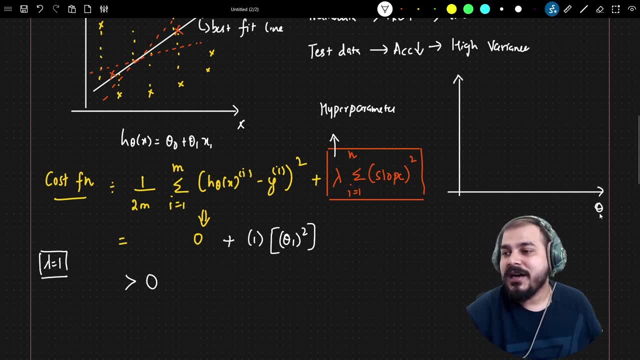 and this specific curve is with respect to theta. that is my slope and cost function is greater than theta and cost function j of theta. Now, in this particular case, if you know that we will be getting this kind of gradient descent right, Let's say I'm just going to put some points over here. 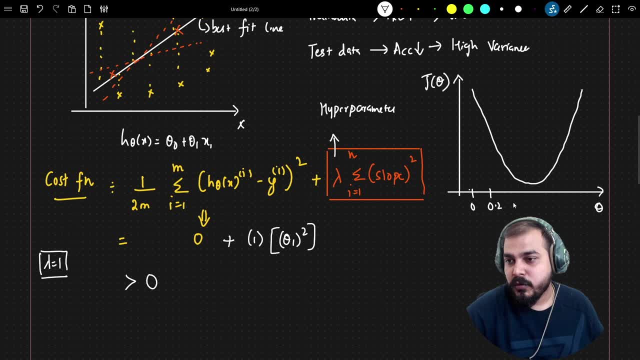 like point. let's say: this is zero, this is point two, this is point four, this is point six, this is point eight, this is one point zero and this is minus point two. Okay, let's say this. I have just plotted. 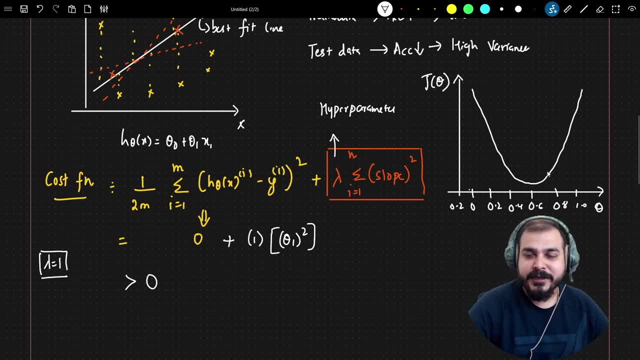 with respect to theta and the cost function. okay, with respect to this gradient descent. Now just to understand when lambda is equal to zero. see, when lambda is equal to zero, that basically means what. I will just have the same linear regression cost function. 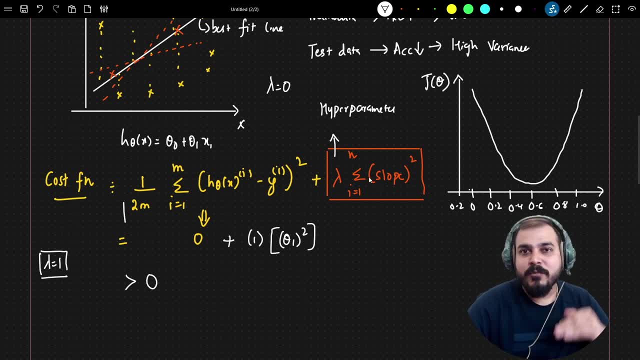 Okay, if lambda is equal to zero, this entire value will be zero. So that basically means I'm not applying ridge regression over here. Whenever I apply ridge regression, I'm basically using this equation at the end, right. So when lambda is equal to zero, 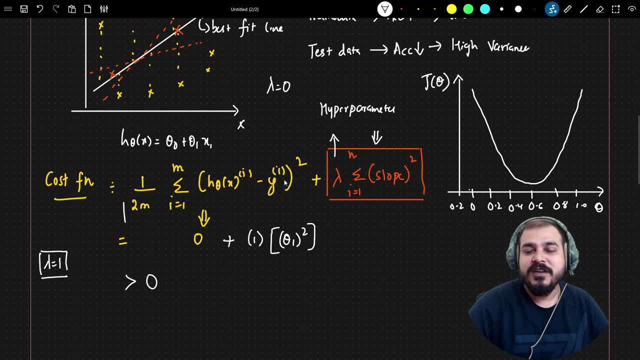 I'm just having this linear regression over here, the same cost function of the linear regression. This is fine. So this is basically my global minima, right? I hope this is my. This is my global minima, So let me say that. okay, this is my global minima, okay. 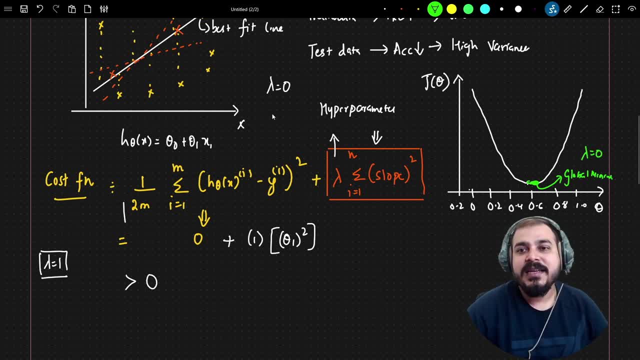 And this is when, When your lambda is equal to zero. Now, let's say, I increase my lambda to 10.. Now, what will happen is that I will get a new line which will look something like this: okay, If you probably try to plot theta, 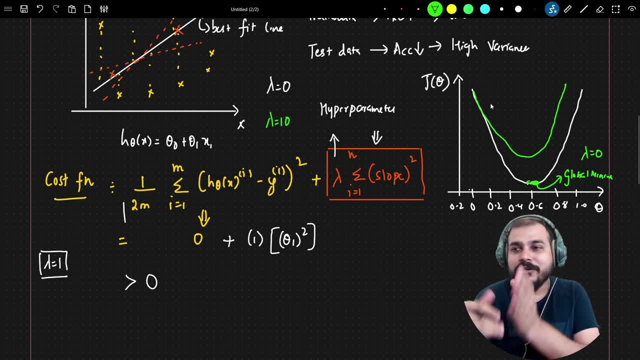 I'm just trying to show you how the plotting, how the graph will look like when we increase our lambda. You can definitely check out by playing with different, different values. Thus you increase the lambda value with respect to this theta right. 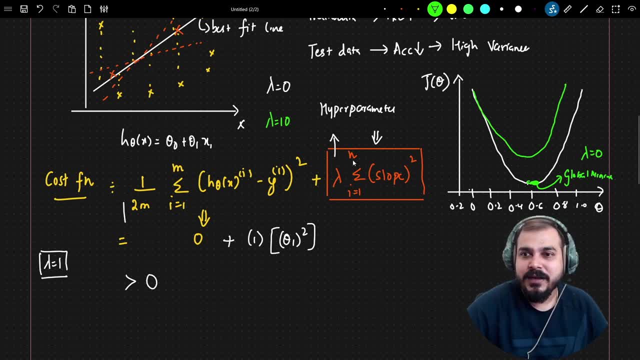 What will happen is that now this lambda value is basically getting assigned some value over here, that is 10, and when we multiply with the slope square, I will be getting a new gradient descent, and now you will be able to see that my global minima has changed. 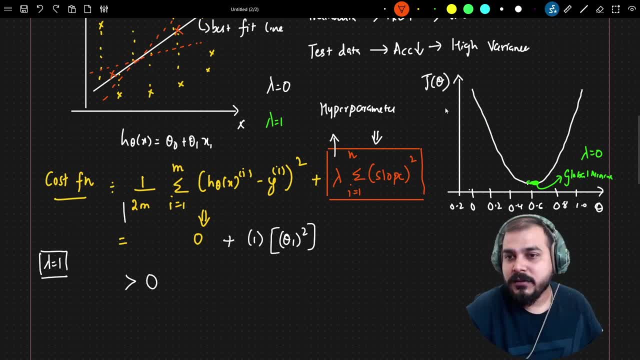 When my global minima has changed. so let me just draw this line properly so that you will be able to understand. So let's say, my lambda is equal to 10.. So what will happen is that when the lambda value increases, I will be getting a new gradient descent. 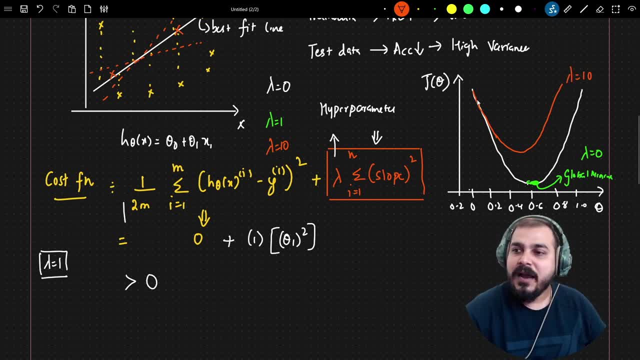 I will be getting another line which looks like this: So during, when lambda is equal to 10,, I'll be getting a different gradient descent. And now, what is the difference between this gradient descent and this gradient descent? Here you can definitely see that. 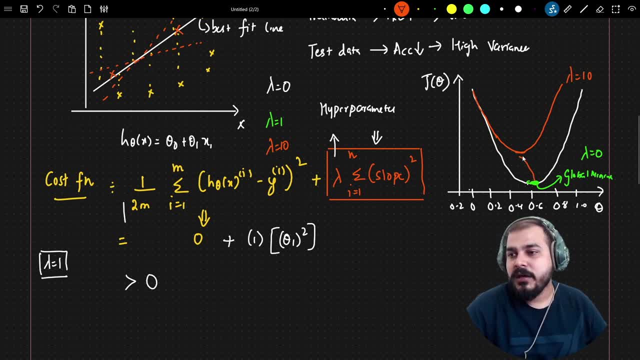 my global minima has shifted. It has shifted from here to here, right? Similarly, my theta value has got reduced. okay, It has basically shifted from here to here, right? This particular is with respect to this theta value. Now, similarly, if I keep on increasing my lambda value, 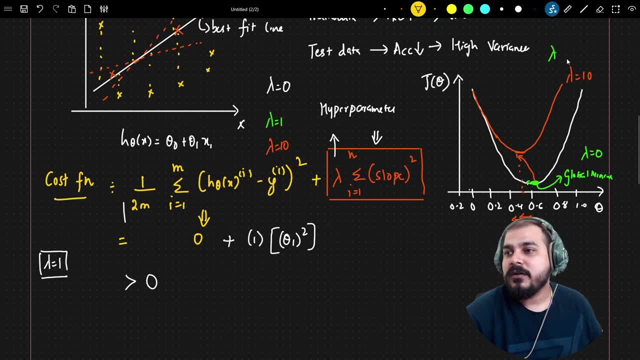 let's say, I increase my lambda value again, so with respect to, lambda is equal to, let's say, 30, then I'll be getting another line which will look something like this: And now this will again get shifted, This global minima will get again shifted somewhere here. 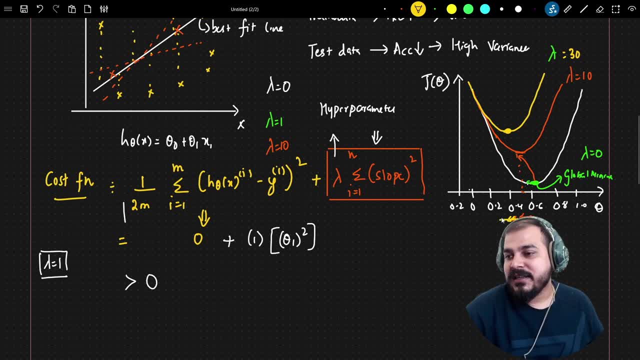 So, in short, what is happening? Theta value is again getting reduced And like this it will keep on happening. but always remember, in this particular scenario, it will never be zero. okay, It will never, never be zero as I keep on increasing the lambda value. 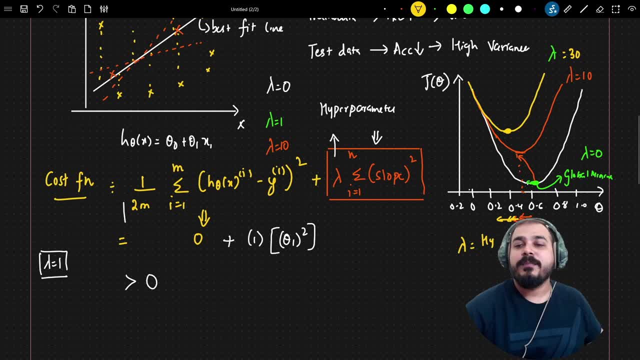 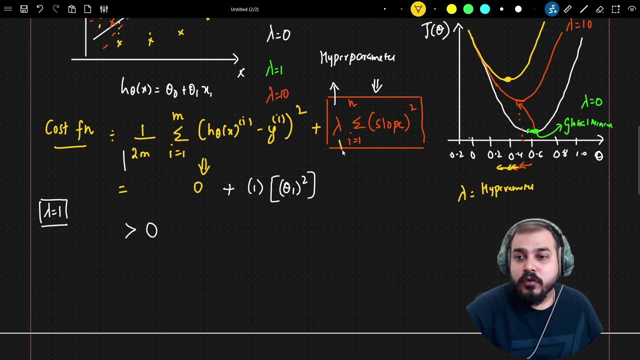 So lambda over here can be considered as a hyperparameter. okay, So lambda can be basically considered as a hyperparameter And if you really want to know the relationship between lambda and slope, you can definitely say: when lambda is increasing, your slope is decreasing. 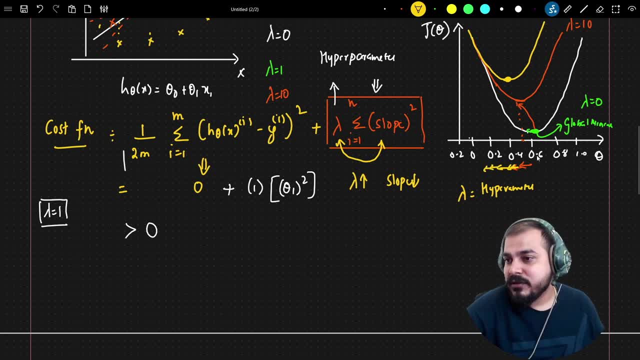 How slope is decreasing Because we are going on this left-hand side. right. You can see, from 0.6, it became 0.4, 0.2, like this it is going on the left-hand side. So this is the exact relationship between lambda and slope. 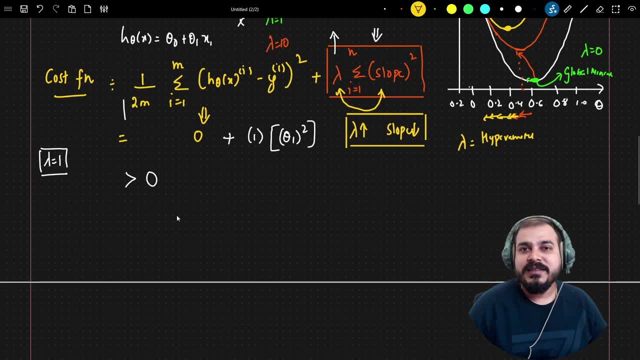 But why we are trying to understand this particular relation. Let's say I have a multilinear regression. okay, Let's say I have a multilinear regression which is like this: theta zero plus theta one x one plus theta two x two plus theta three x three. 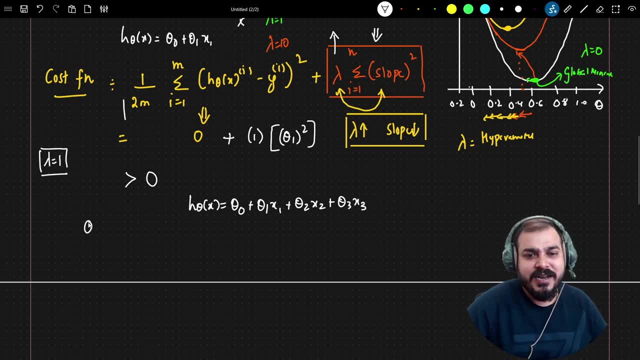 Let's say I have three coefficients and three independent feature, And let's consider that theta zero is equal to zero. If I say theta zero is equal to zero, then what does this basically indicate? This basically indicate that it is passing through the origin, right? 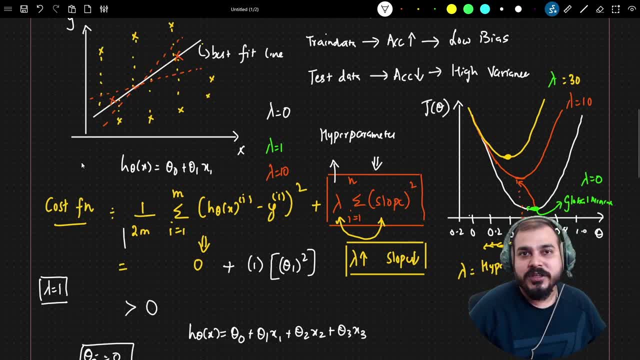 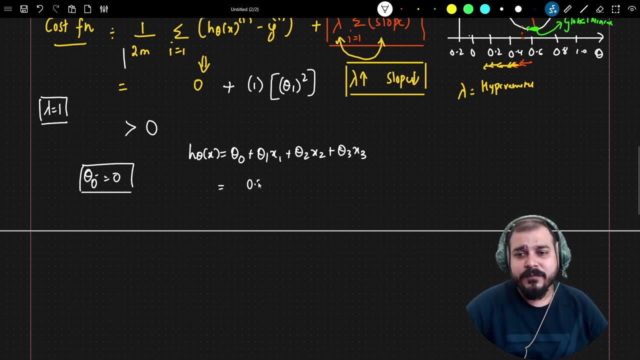 The specific line. this line is basically meeting the y-axis in the origin. This I have already discussed. Now let's consider that my theta one value- I'm assuming, okay, I got somewhere around 0.5- to x one, I'm just assuming theta one. theta two, theta three: 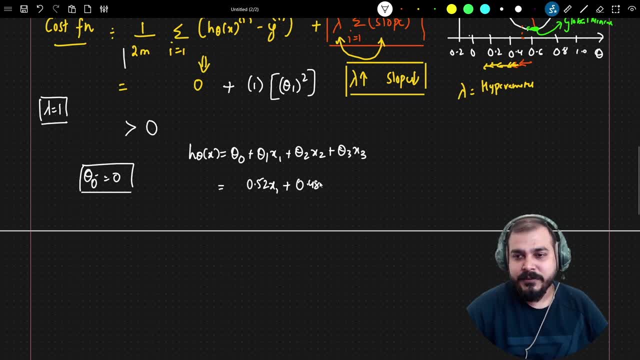 Let's say, over here I got probably 0.48.. And here I got probably 0.24, x, three right Suppose. I got these values and obviously I have theta zero as zero. If I don't want to even take this, 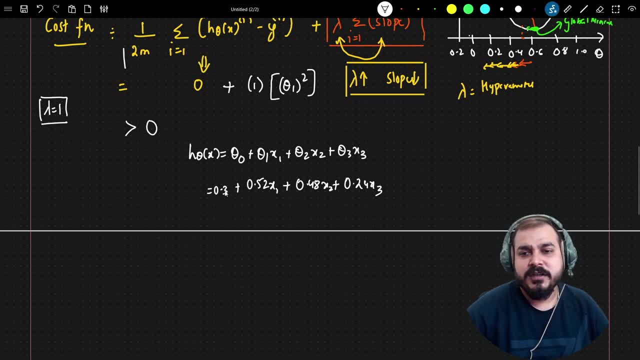 let's consider some different theta: zero value. So let's say this is 0.34.. My intercept is 0.34.. Now, in this particular scenario, what will happen is that if I apply ridge regression on this cost function, then this value will get reduced. 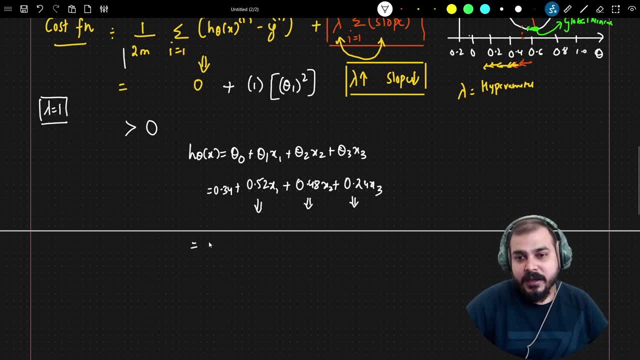 This coefficient will get reduced, but it will never be zero. See what does this value basically indicate? 0.52 of x one. This basically indicates that, with the unit movement in x one, right With the unit movement in x one. 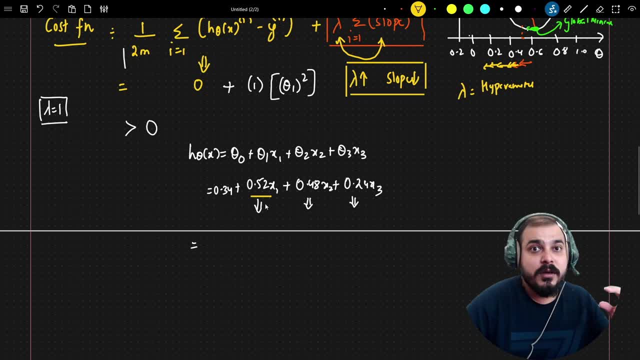 what is the movement with y right? So here you can see 0.52 movement with respect to y. Similarly, with the unit movement with respect to y right, With the unit movement with x two, what is the unit movement with respect to y? 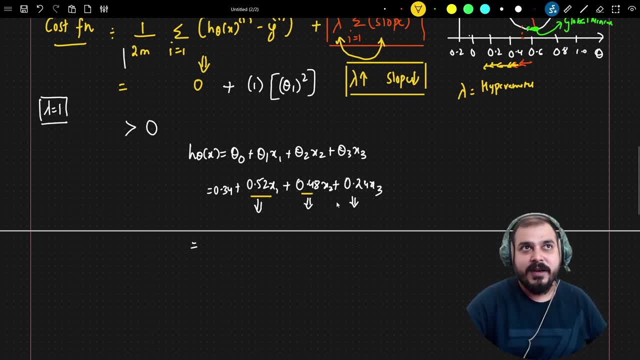 So here you can see that it is 0.48 unit movement with respect to y. I'm not saying unit movement, but 0.48 movement with respect to y. That basically means if x one is moving by one, then y will move by 0.52. in this particular case, 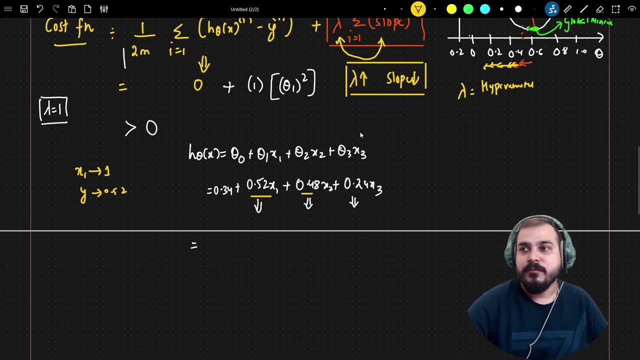 If x, two is moving by one, then 0.48 y will basically be moving right. So this is what it basically indicates. Now, if there is too much movement with respect to unit movement, if there is a unit movement, that basically means these features: 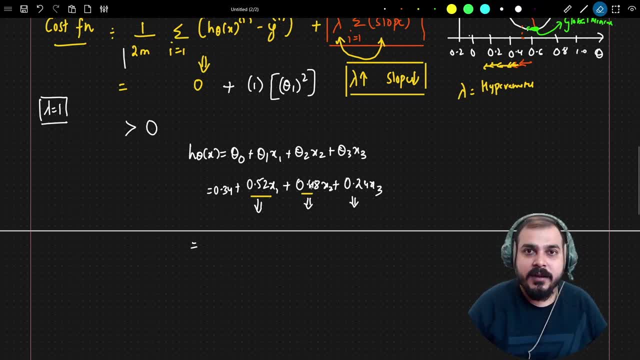 are highly correlated with the output feature. right, Highly correlated with the output feature. But here you can see that with respect to x three, we have a very small value: 0.24, right, Even though we have a very small value. 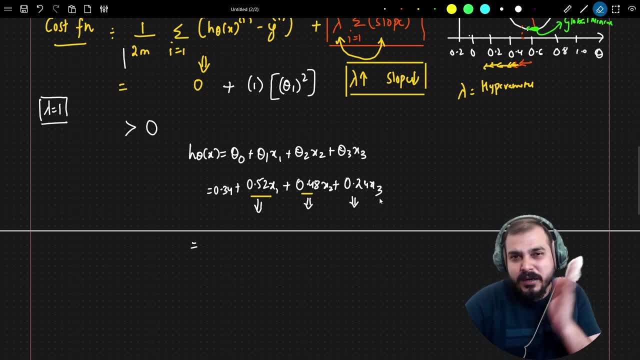 what will happen is that if I try to make a movement unit movement with x three, there'll be a small unit movement with respect to y right, Somewhere around 0.24.. But when I apply ridge regression to this equation, 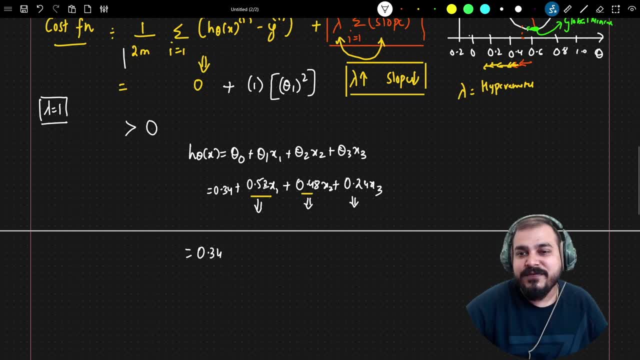 I may get something like this. See, I may get something like this, where this value will get reduced. This value will get reduced, Let's say it will get reduced to 0.40 x one. This may be 0.38 x two. 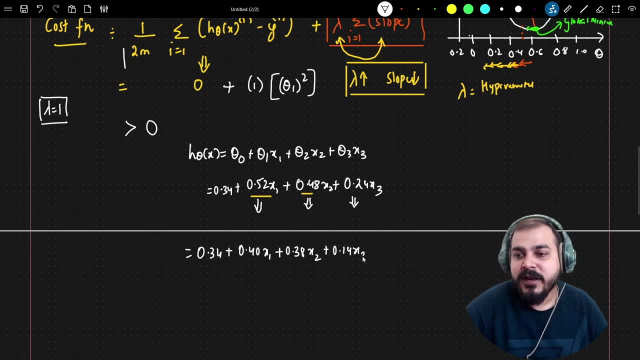 But when I see this value, this value will also get reduced 0.14 x three. But here you can see that, since this value has now a very small coefficient, this won't impact much change in the movement of this specific line. okay, 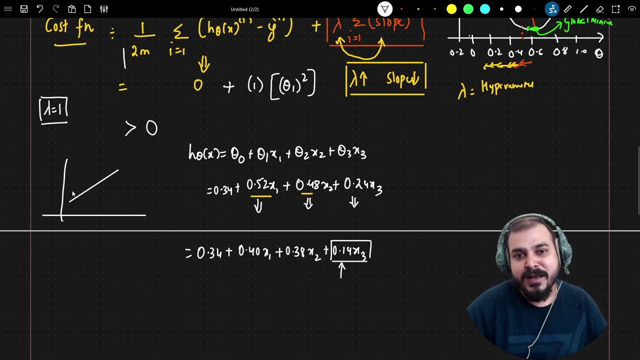 Because in this particular case, I have three coefficients, So this will then become a plane. This may become a plane entirely, right, The line that we are specifically using for division, right? So here you can see over here, since this value is very, very small. 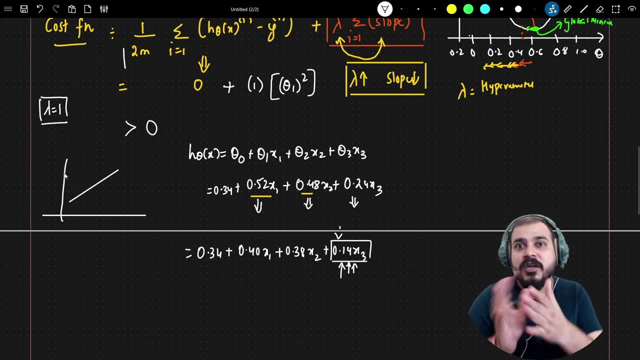 this won't impact the best fit line by a major movement. Only a smaller movement will basically happen And always remember this value will never become zero. That is what ridge regression basically does And how it is reducing overfitting, Because it is reducing the impact by the coefficient right. 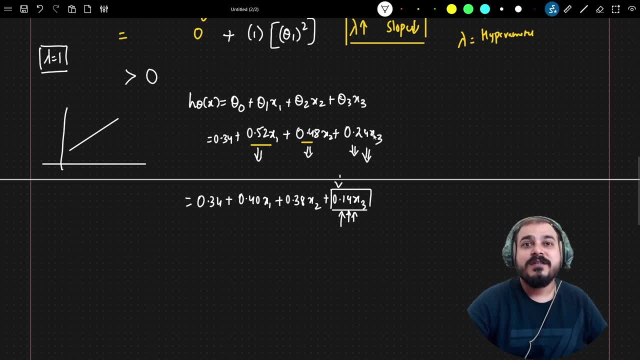 Because it is reducing the impact by the coefficient right, Because it is reducing the impact by the coefficient by reducing the coefficient of the feature that are not directly correlated with the output feature. Now, here you can see, x three is hardly correlated by 0.24.. 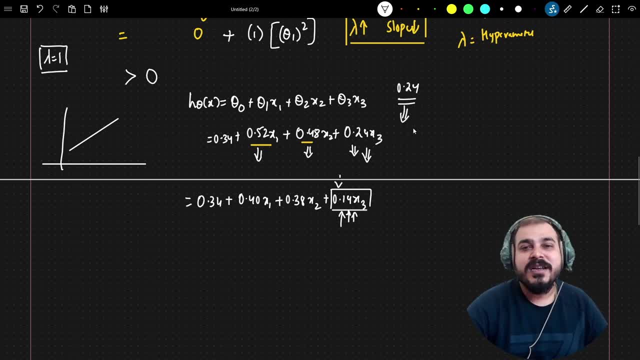 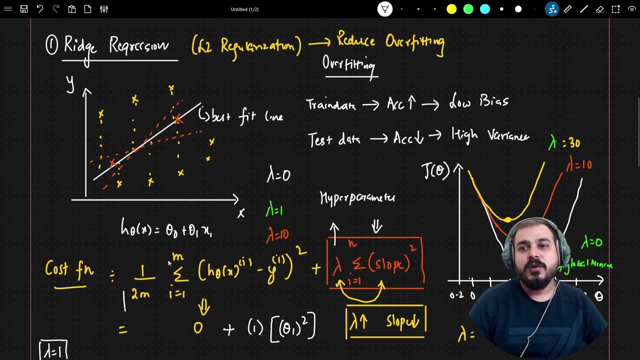 And it is trying to reduce this particular value also, And when it reduces this particular value, that basically means this will not have much impact on the best fit line, right? So I hope you are able to understand. I hope you are able to understand the relationship. 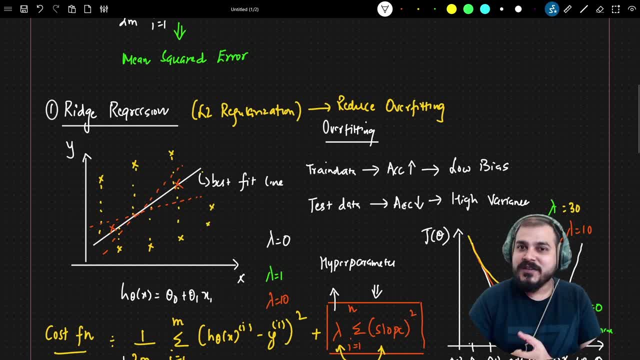 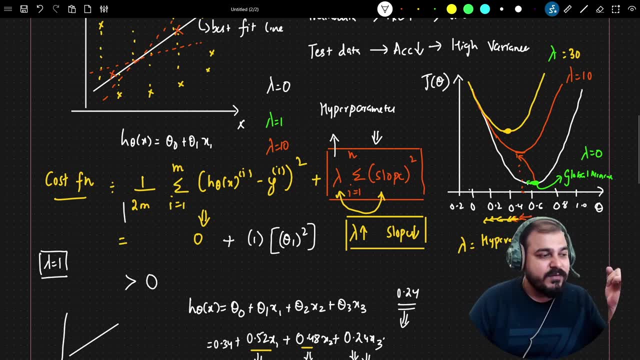 between lambda and slope. So please just try to go through this video again. This is all maths you really need to know, guys. Then only you'll be able to understand what things are actually happening. Now, in the next video, we are basically going to discuss about 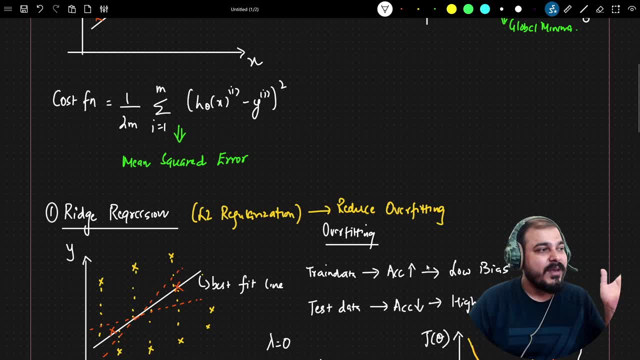 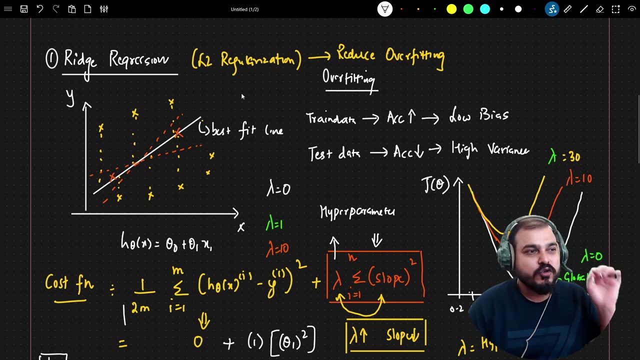 something called as lasso regression. So right now we have completed ridge regression. We have already understood about ridge regression, which is also called as L2 regularization, And a super important interview question may come that: why do you use ridge regression? You basically have to say about it: reduces. 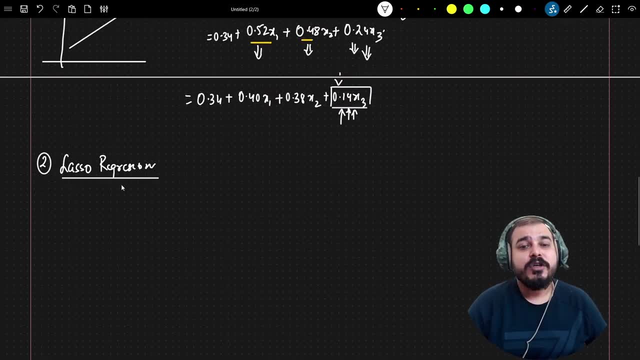 it is basically used to reduce overfitting. Now in this video, we are going to discuss about lasso regression, And lasso regression is also called as something called as L1 regularization. And why do we specifically use? We specifically use for a very important work. 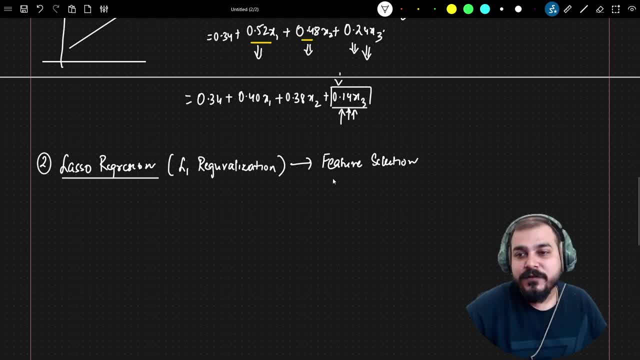 that is called as feature selection. Now how do we do feature selection and all? Let's discuss about this Now in lasso regression. we just need to focus more on the cost function. So here the cost function is nothing, but it is one by two m. 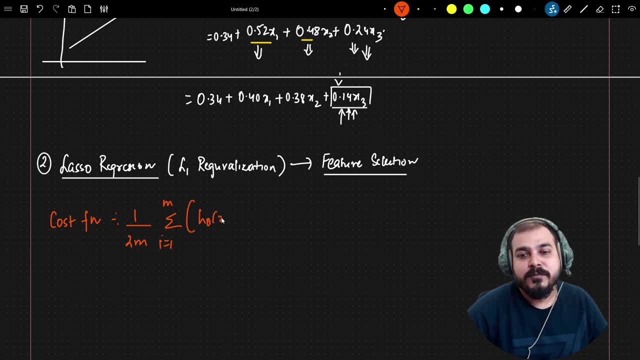 and the sum of m is equal to m. And here, obviously, you have something called as h, theta of x of i, which is my predicted point y of i. Along with this. now we are going to add two more parameters. One is lambda. 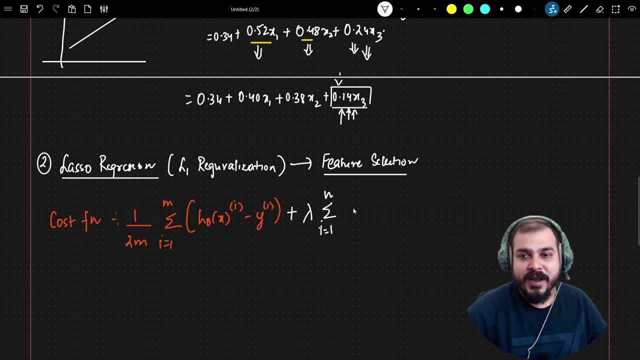 and the second one is something called as summation of i is equal to one to n, not slope square, but it should be magnitude of slope. Now, with the help of this specific equation, we will try to do some feature selection. Feature selection basically means: 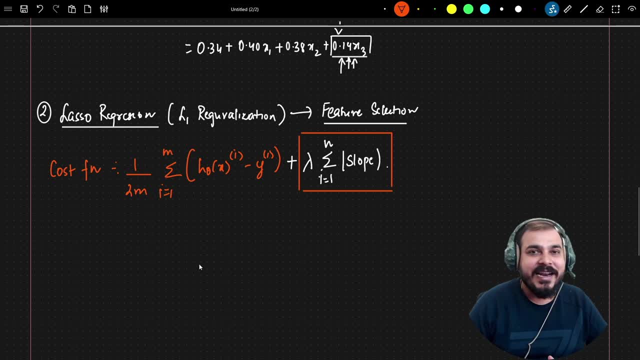 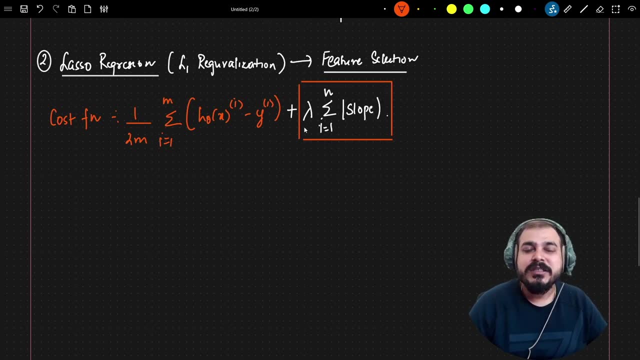 the features that are not in the picture, the features that are not that important will automatically get deleted, And features that are very, very important, it will be considered. Now if I try to show you the relationship between lambda and this slope, okay, 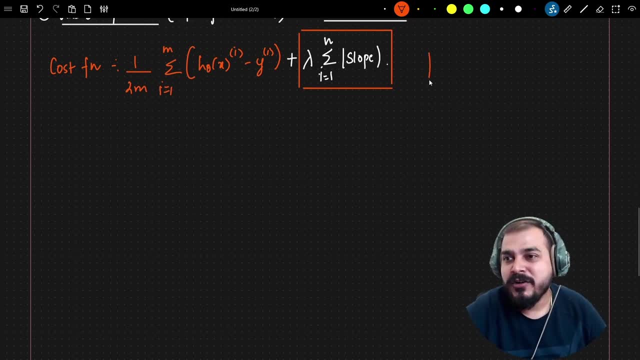 with respect to this specific cost function. So suppose, if I try to draw this cost function over here in the right hand side with respect to theta and j of theta by using this cost function, obviously the first one if your lambda value is zero. 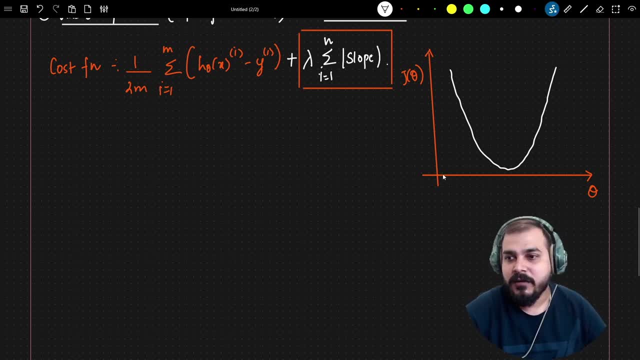 I will be getting a normal curve right, Normal gradient descent curve. So let's say this is my zero. So let's say this is my- I'm just going to use this over here- zero. This is minus 0.2,. 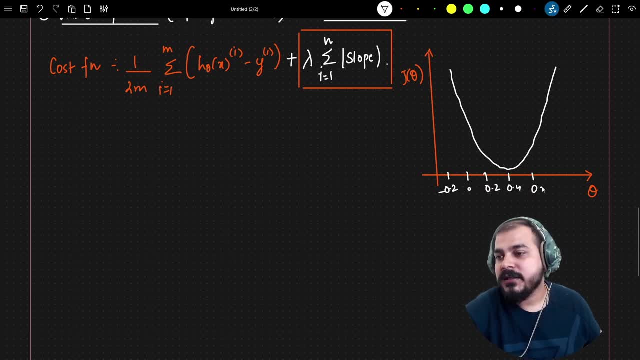 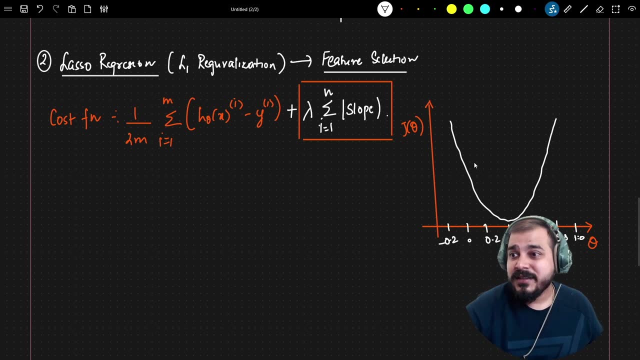 and this is 0.2, 0.4,, 0.6,, 0.8,, 1.0, okay. So if I try to draw this kind of curve, this curve is called as gradient descent curve, With lambda is equal to zero. 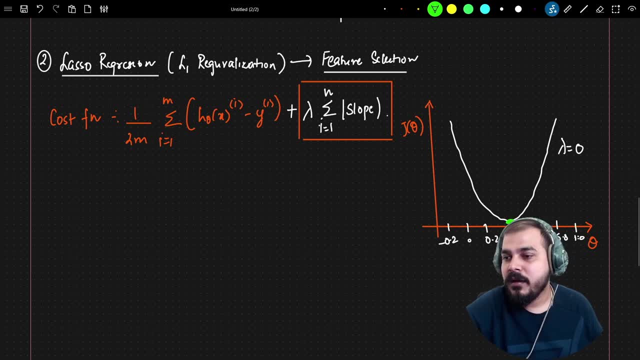 I'll be getting this kind of curve right, And this is obviously my global minima. So what happens when my lambda value will increase? Then I will probably get my another curve, which will look like this. okay, And let me just draw this. 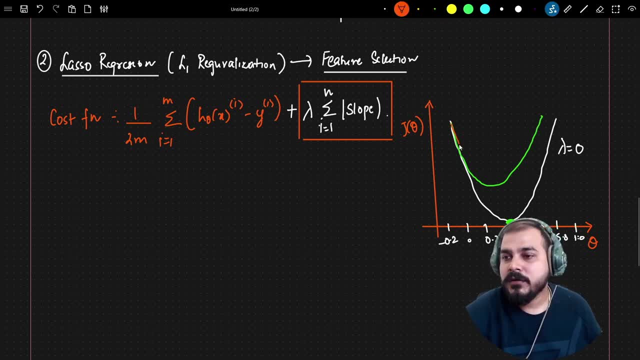 and then everything will make sense. okay, And then I may probably also get one more curve which may look like this, And, finally, I may get one more curve which will look like this, which will look like this. okay, Now, what is the difference between this curve? 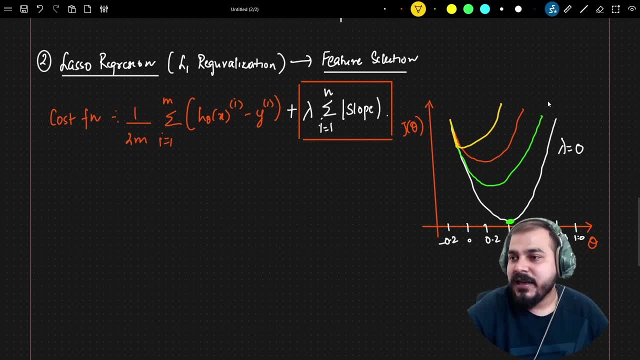 and the previous curve, when my lambda value is increasing. Let's say: this green line is basically when lambda is equal to 10,, this is lambda is equal to 20,, this is lambda is equal to 40,. let's say: okay. 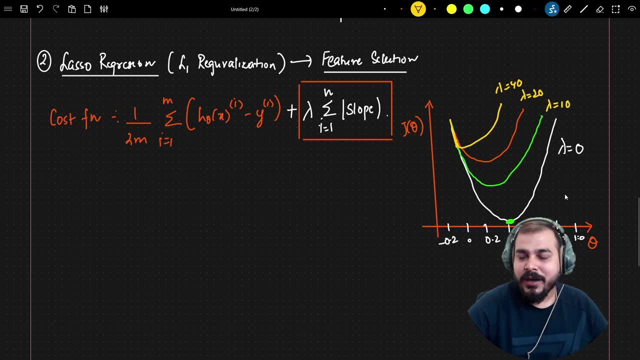 Now, in this scenario, what happens is that, obviously, as I increase my lambda, my theta value is decreasing, But you will be seeing that after one point of time, my theta value will become zero. okay, So this is nothing, but this is basically becoming zero. 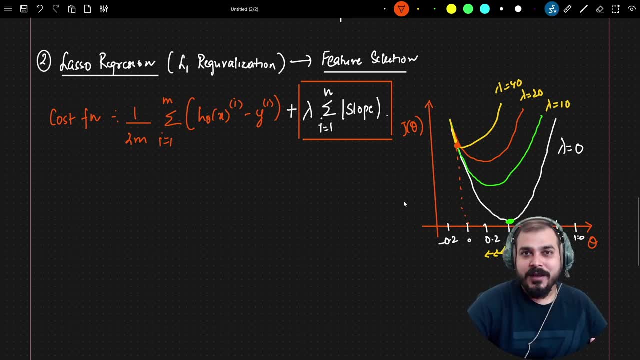 So, in short, my coefficient is actually becoming zero. Now, what happens if my coefficient actually becomes zero? In short, we are actually, but we are actually trying to remove that specific feature, right? So let's say, my h theta of x is this specific equation. 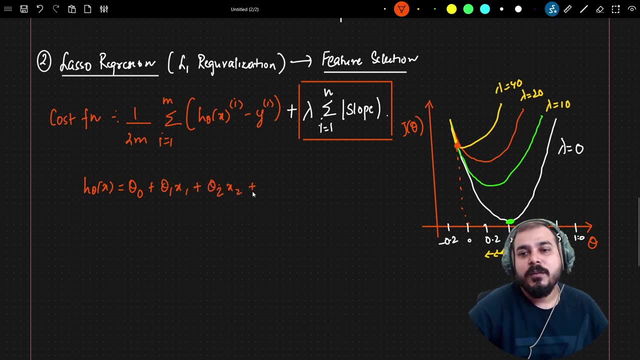 theta zero plus theta one x one, plus theta two x two, plus theta three x three, plus theta four x four. Let's consider that I have four independent features. Let's say my theta zero is 0.52.. My theta one that I have probably computed- 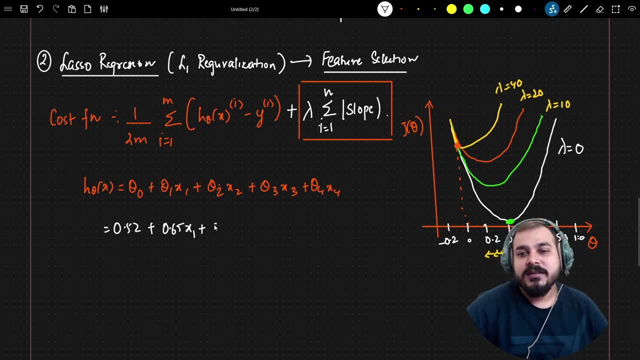 by creating the best fit line is somewhere around 0.65 x one. This is 0.72 x two. this is 0.32 x two. This is 0.34 x three, unless this is 0.12 x four. 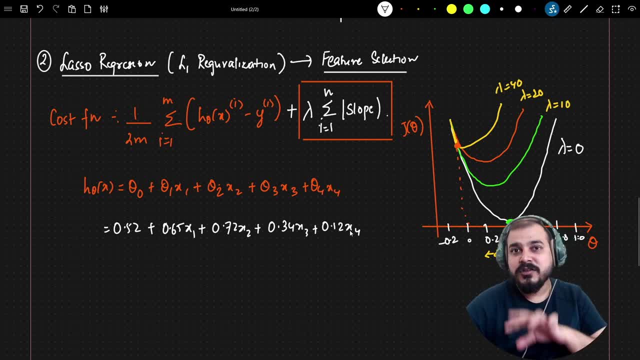 Now, in this particular scenario, you can see that x four is the feature that is not much correlated with the output feature, that is, with respect to h theta of x, Because here why We have a very small coefficient, that is 0.12.. 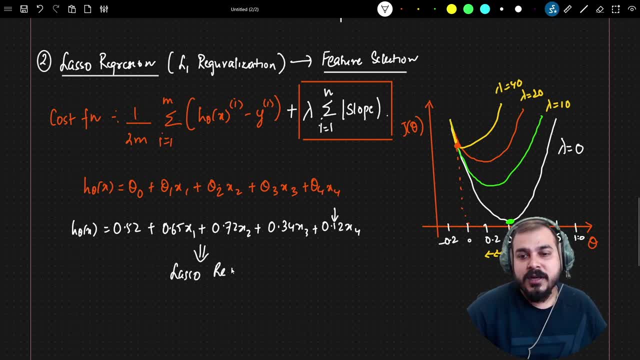 So, after we apply over here lasso regression- since this feature is not that important- what it will do is that it will try to reduce this entire. it will try to reduce this coefficient to something, Something like zero. So zero multiplied by x four will actually become zero. 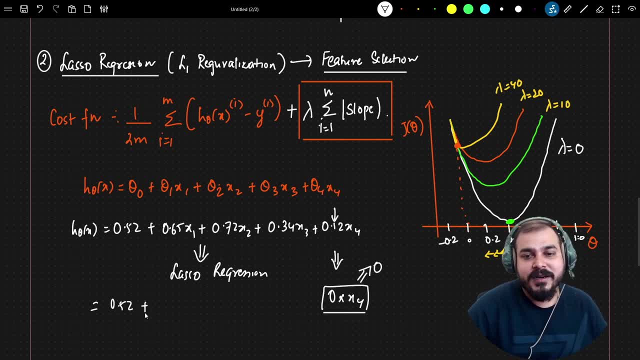 So this will entirely become zero And this all value will get reduced by a smaller number: five one x one, because this is directly correlated. So this may be x two, this may be 0.14 x three, like this. So in this way, you can see that this feature. 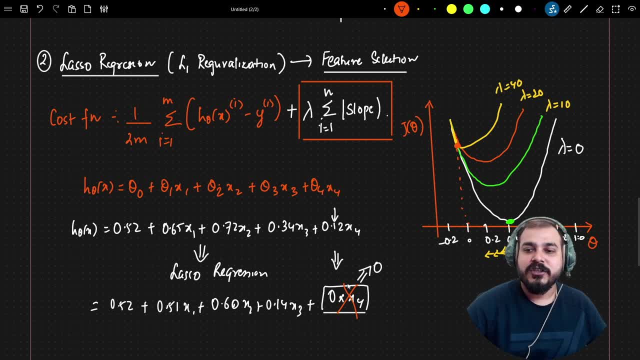 is being removed and we have not used this particular feature, or this coefficient has become zero because this feature is not that important. So this is what basically indicates: once we add this specific term in the cost function, right, Once we add this specific term in the cost function. 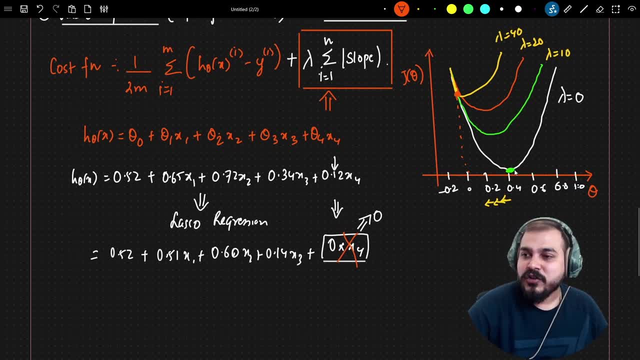 we can see that. what is the relationship between lambda and slope? So here, obviously, your theta value is becoming less, but at one point of time this will become zero. That is, your theta value will become zero. So the same thing is basically happening over here. 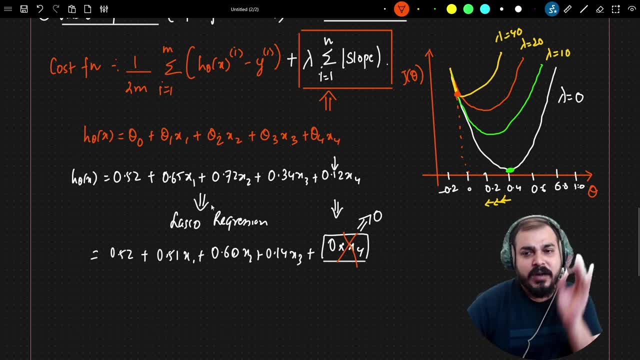 which all features are not that much correlated. And if it is not correlated then obviously it will be having a small coefficient value. but if it is not correlated then obviously it will be having a small coefficient value. So after we apply lasso regression, 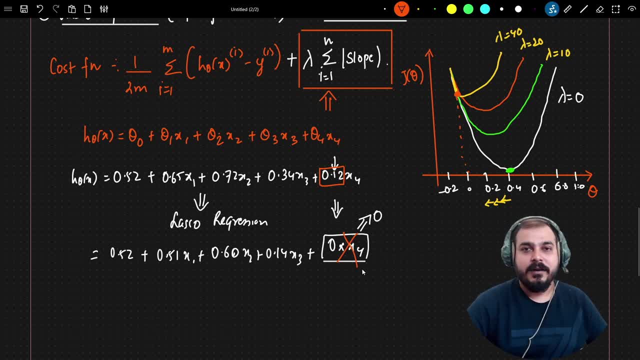 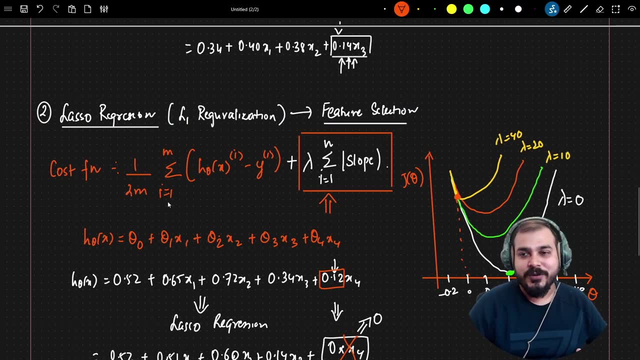 this will actually become zero And by this, this entire feature is getting removed and remaining. all features is basically used to find out the best fit line, right. So this is the importance of lasso regression, right, And when we do use this. 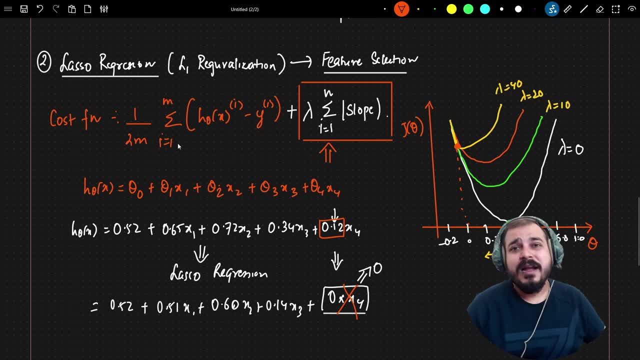 suppose if I have hundreds and hundreds of feature right, I should definitely go ahead and use lasso regression because automatically it will be able to find out features that are not that highly correlated. It will just try to remove it because it is going to make the coefficient to zero, right. 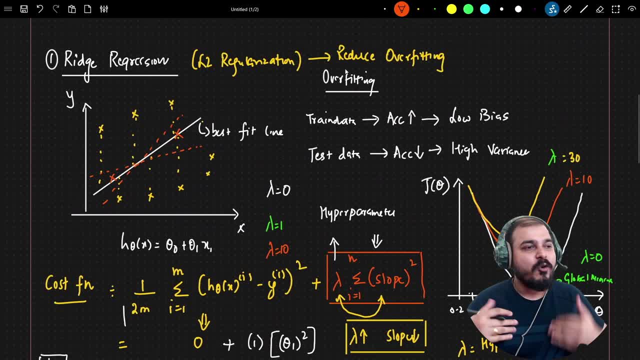 Similarly, when should we use ridge regression? It is very simple: Whenever overfitting condition basically happens. when your training data accuracy is very, very high and your test data accuracy is very, very low, this, basically, is an overfitting condition. 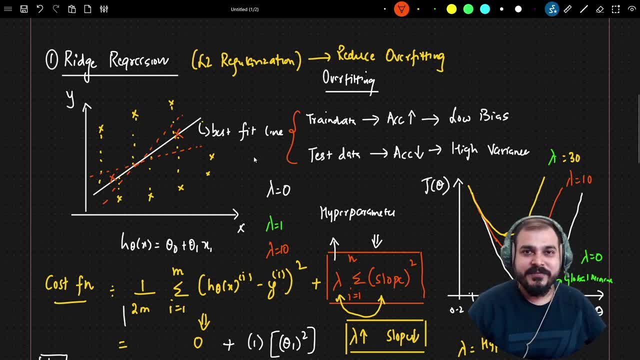 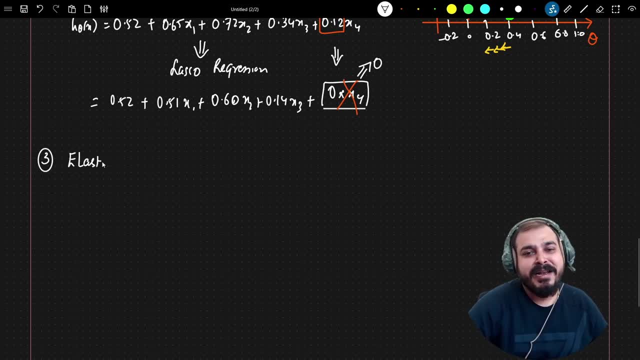 So we should basically try to apply ridge regression in this particular case right Now. coming to the next one, which is super, super important: What is elastic net? right? Elastic net is nothing, guys. It is the combination of both. 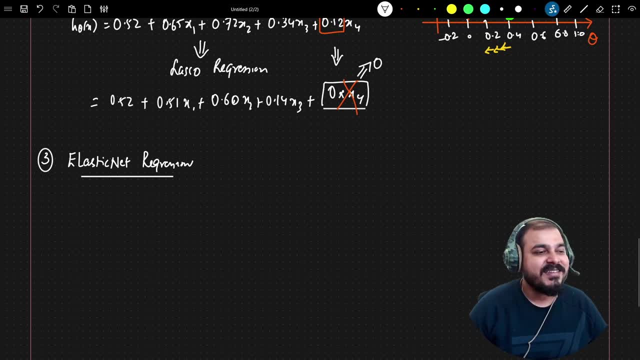 So let me write this With respect to elastic net: it is the combination of both. So let me write this With respect to elastic net: it is the combination of both. So let me write this With respect to elastic net: it is the combination of both. 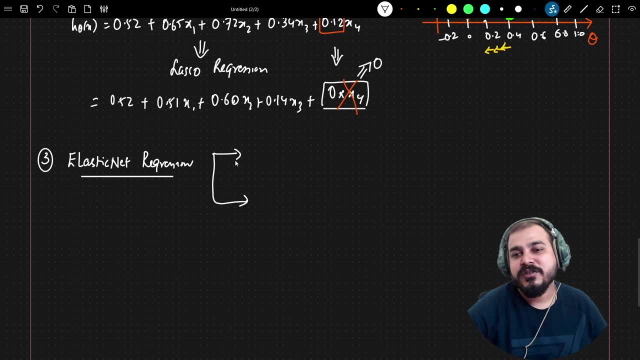 Ridge and lasso. So here, with the help of elastic net, what all things we do? First of all, we try to reduce overfitting, And the second one is that we try to along with overfitting what we do. 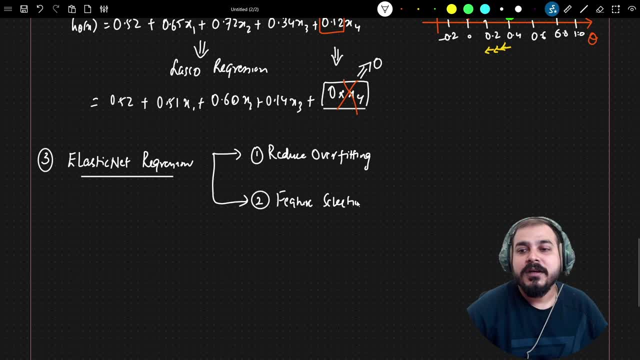 We also do feature selection. So if I combine both ridge and lasso together, that actually becomes a elastic net. So what will be the cost function that may look like over here now? So I may basically write my cost function, which will look like this: 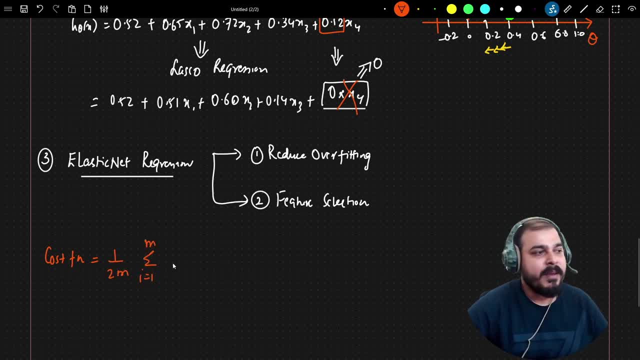 One by 2m, summation of i is equal to one, 2m, And this will be Y of i minus Y of i. I'll not say Y of i, but I'll say h theta of x of i minus y of i, whole square plus. 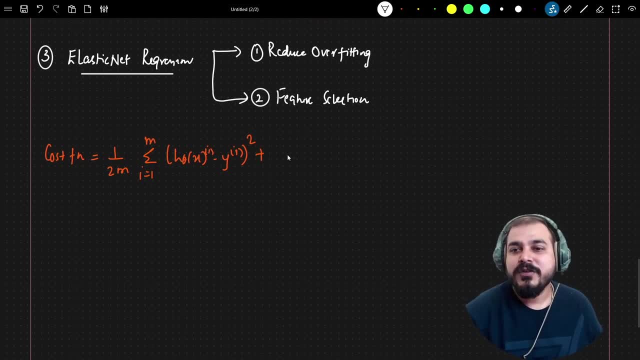 And we can basically use For reducing overfitting. what do we use? We use lambda ones, And this lambda one we can basically multiply with summation ofías equal to 1, 2n, And this will be my slope square.